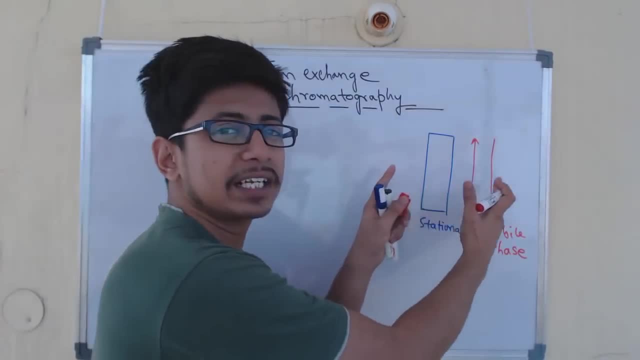 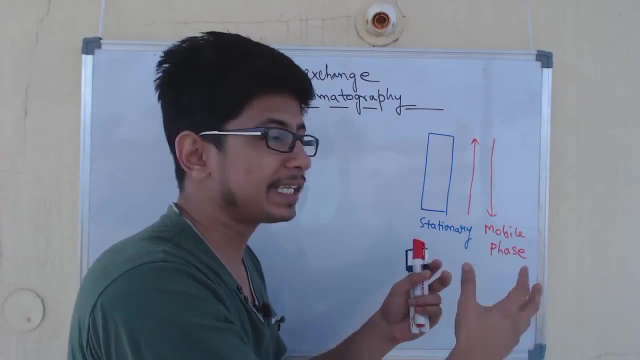 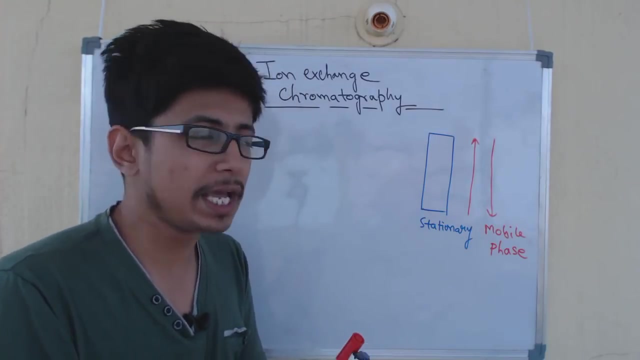 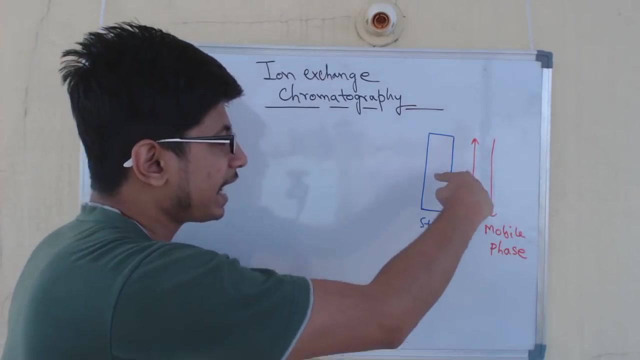 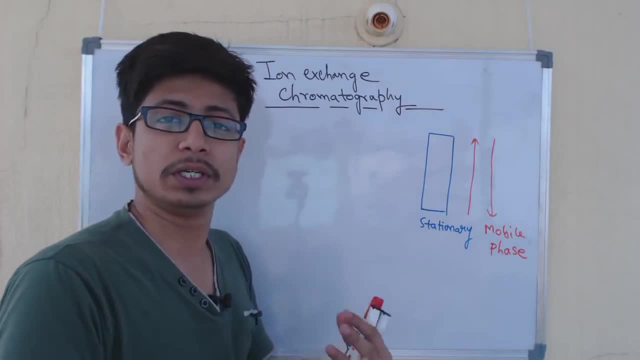 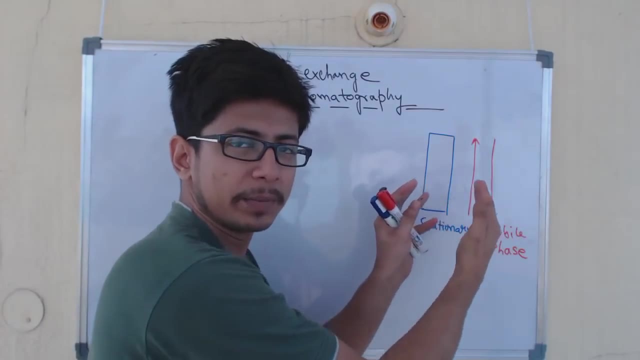 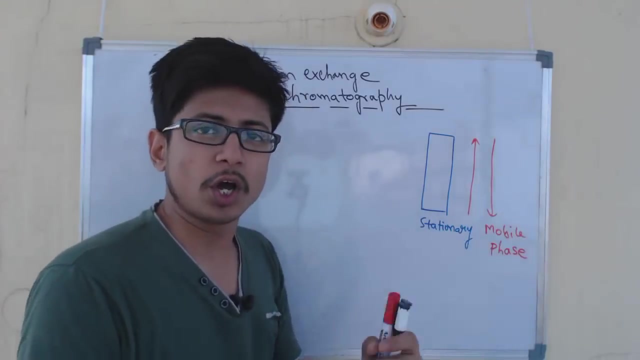 certain molecules to elute and come out fast. certain molecules to elute letter. That is the actual concept of chromatography techniques. It's the phase separation methodology that we use in case of ion exchange chromatography. What kind of molecule we separate? ions or 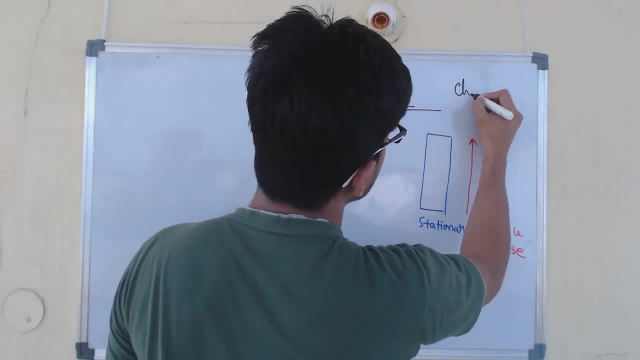 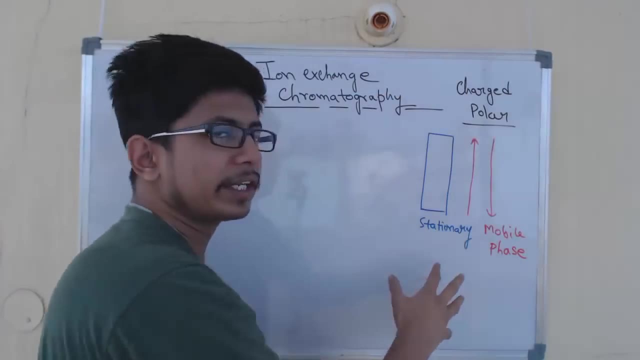 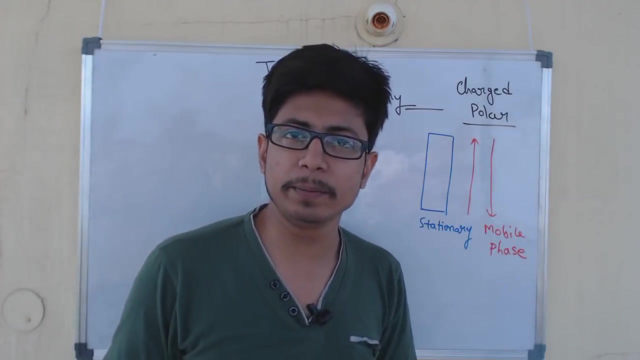 polar or charged molecules. So we always go for charged or polar molecules in this case. Now, in this case of ion exchange chromatography, we run a column. You know, we also talked about column chromatography, but column chromatography means we prepare columns. in its structure 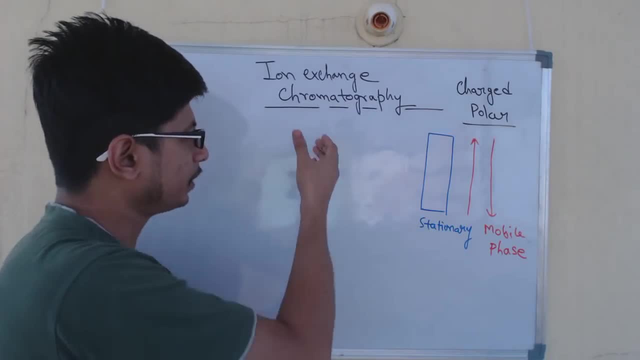 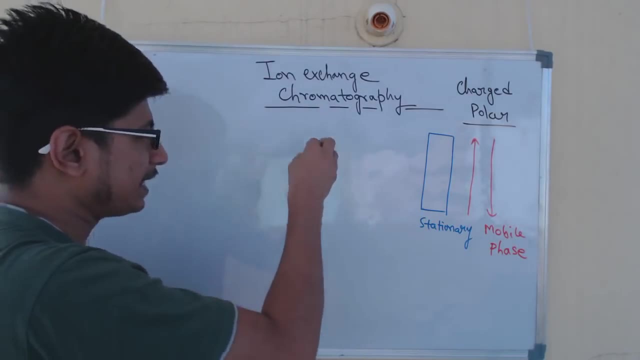 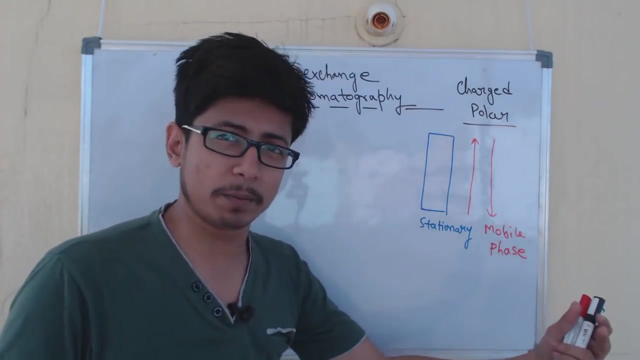 made with polymers, either could be of glass or it could be of any of fiber polymers. that creates a chamber. inside the chamber We add the stationary phase. stationary phase can be of different molecules. Those are polymers, Like cellulose, like you can use your agarose. So those are the molecules which are polymers. 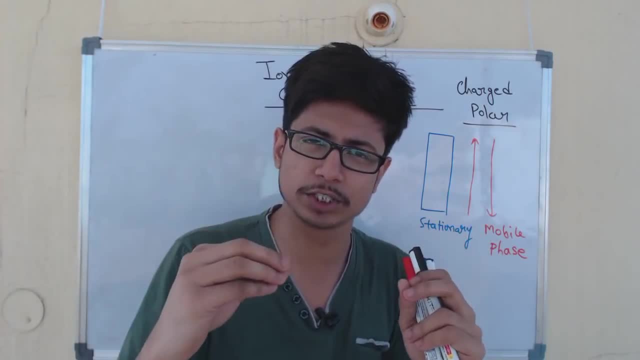 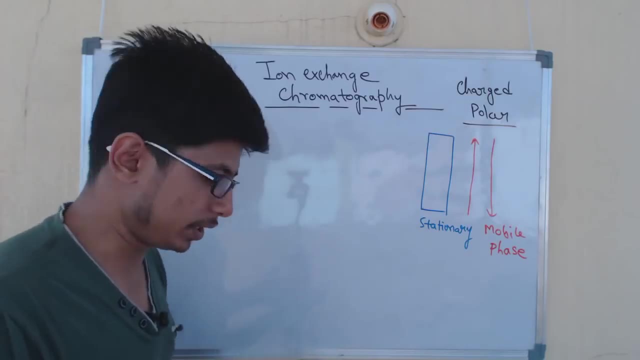 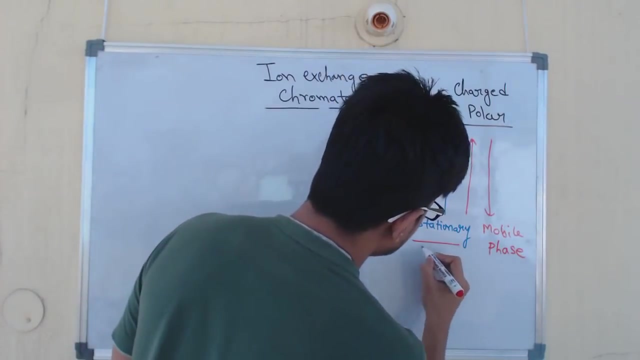 and the polymers actually can create networks and mesh like structures where all the other molecules can move through those networks. So that's why we need this stationary phase as polymers. Now, in this case of ion exchange chromatography, the stationary phase that we use is- it is, in this case, either cellulose or agarose. 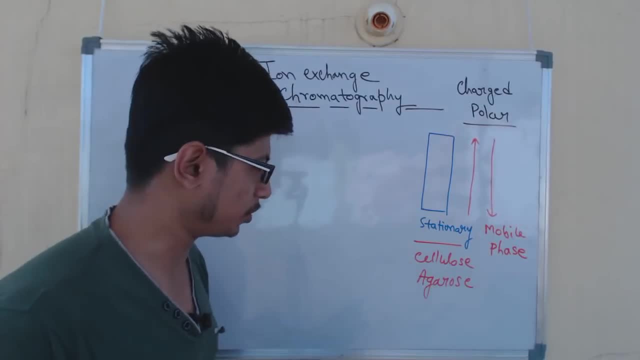 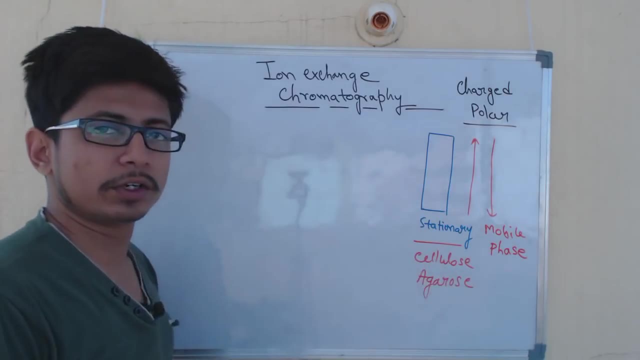 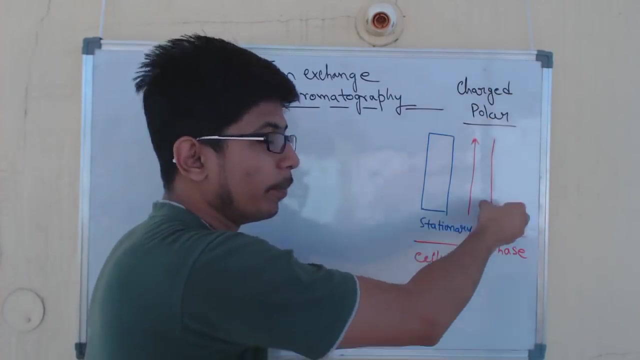 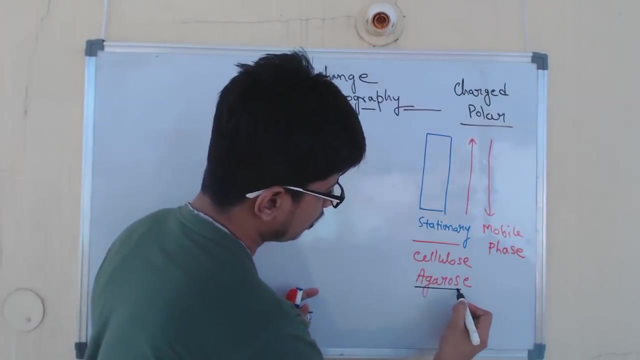 Now, in this case of ion exchange chromatography, the idea is the exchanging this charged or polar molecules from the mobile phase, because here the stationary phase is solid, which is say agarose, for example. This is solid, while the mobile phase Here is liquid. So 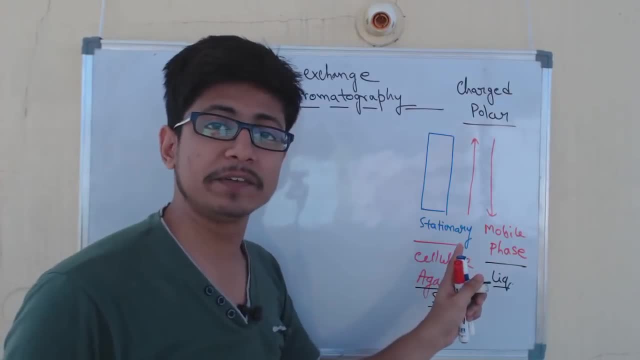 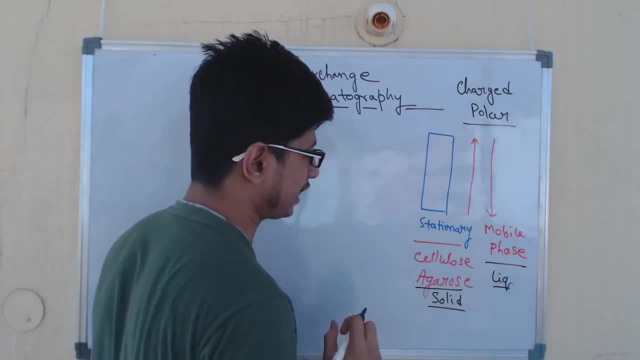 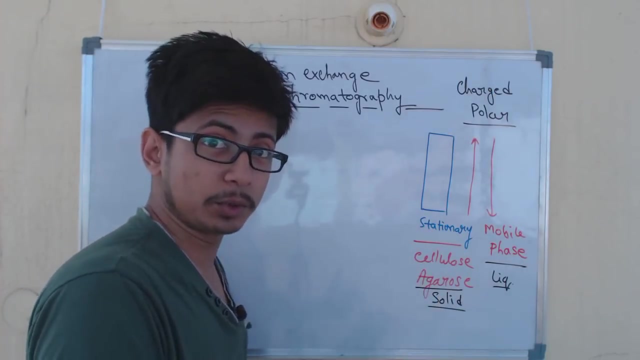 remember this to face can be of different type, like it could be liquid or gas, ok, but here the stationary phase is solid, the mobile phase is liquid. now the liquid contains all other molecules. among them we have the charged molecules and polar molecules that we want to separate from each other, and in this case we have agarose. so what we do here, we take 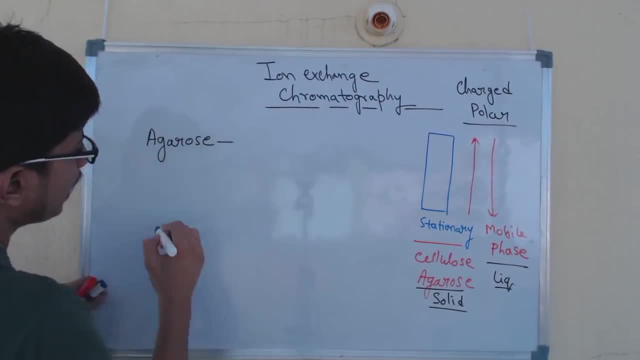 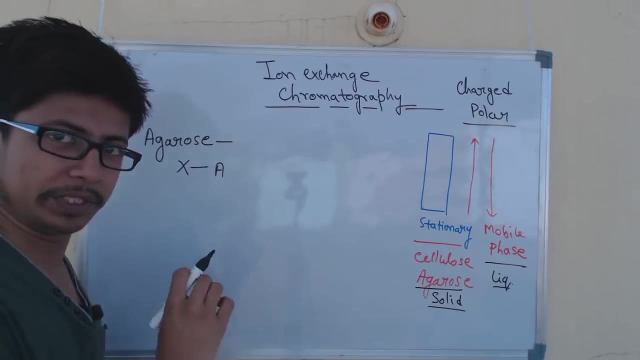 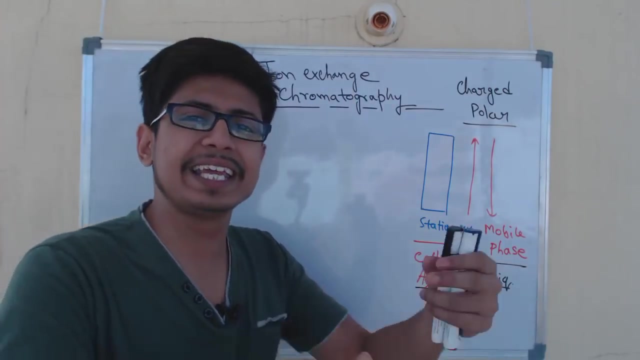 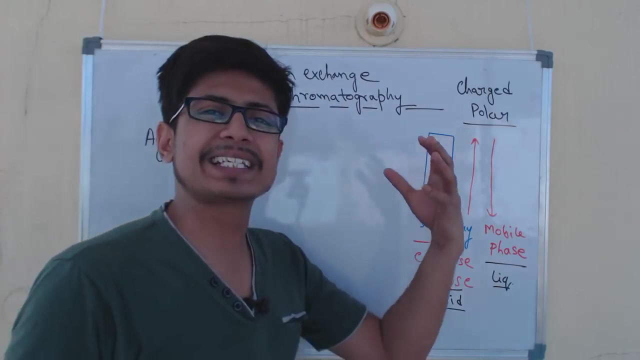 this agarose, and let's assume this as X, and we attach ion with it, some sort of ion or charged molecule with it. now, the idea of ion exchange is to exchange a specific polar molecules. ok, now there are two different types of ion exchange: chromatography. one is the cation. 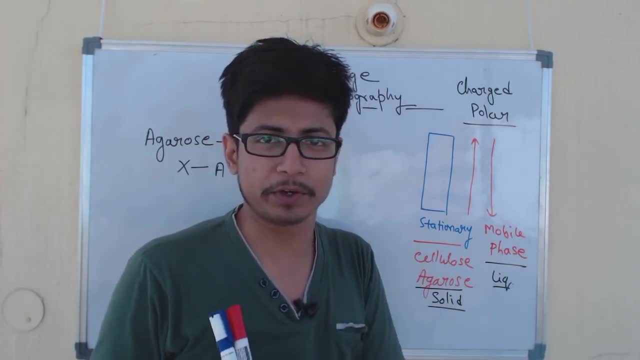 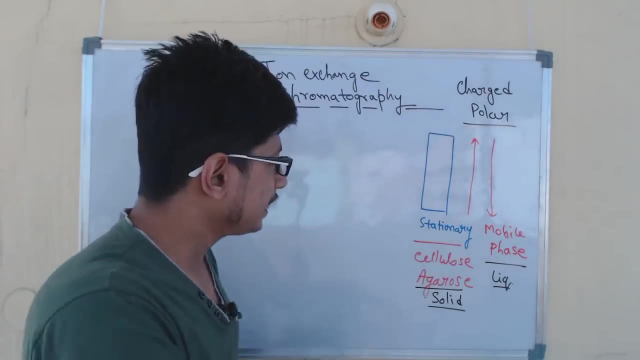 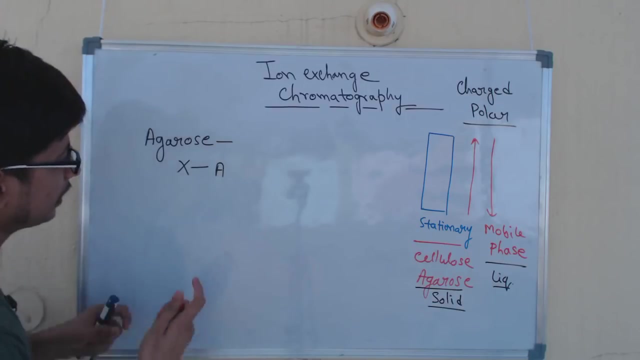 exchange chromatography. another one is the anion exchange chromatography. in the cation exchange chromatography they retain cation. in the anion exchange chromatography this column retain anion. that is the idea. that means the stationary phase is fixed. this is the stationary phase. this is the fixed stationary phase and if it is a cation exchange chromatography. 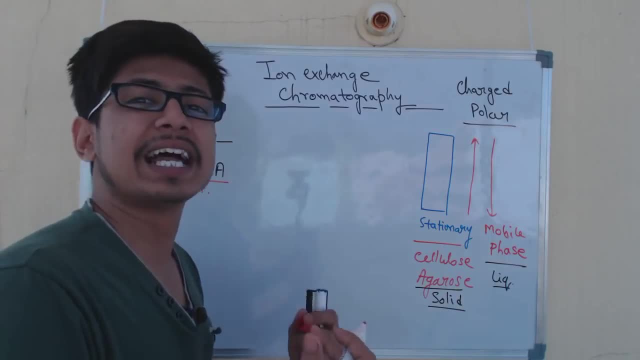 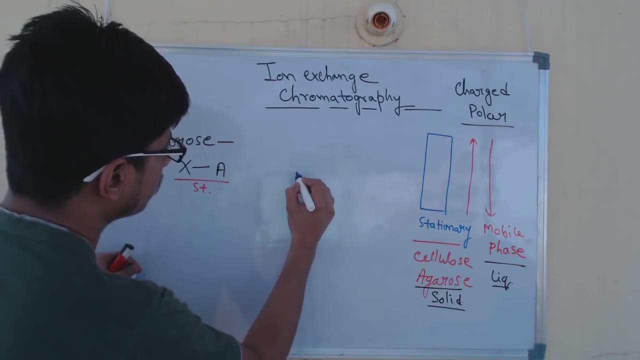 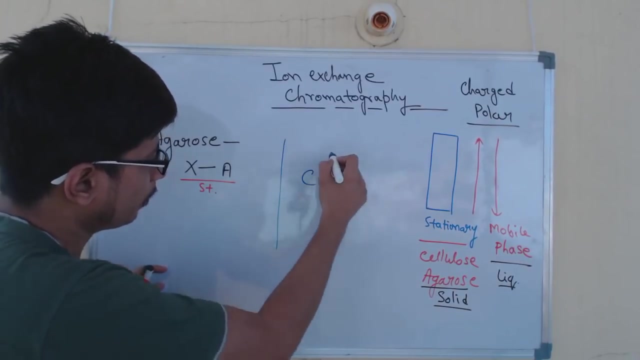 in that case, this will attach to a cation. ok, let's say cation means positively charged ions. Now let's say here: C is the molecule that we want to separate from the mixture. it is in the mobile phase. remember, this is in the mobile phase. ok, and this is in the stationary. 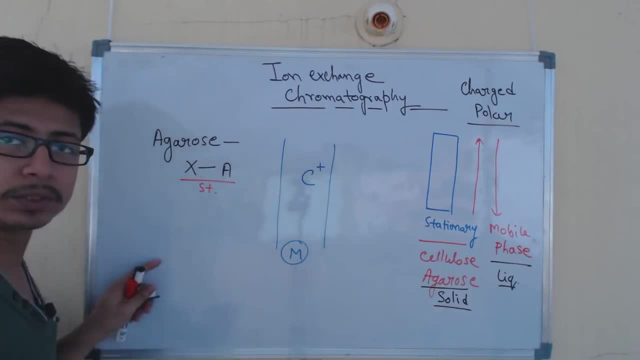 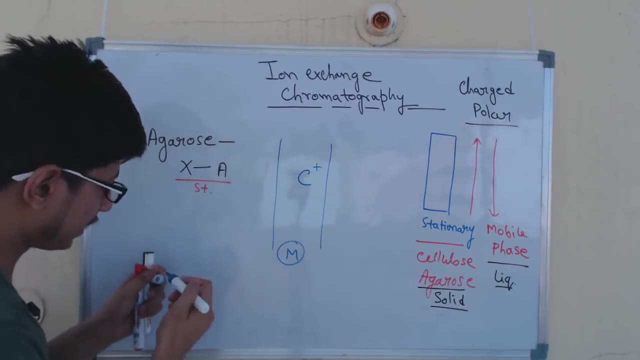 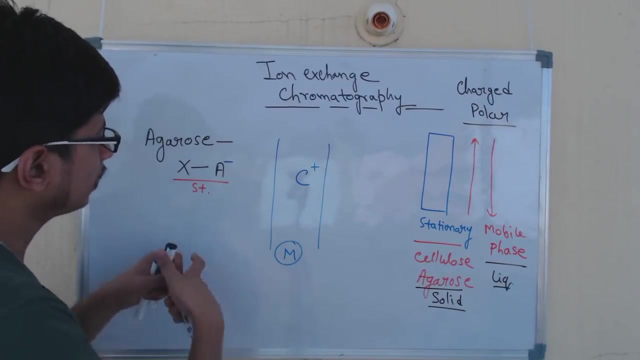 phase. now C is positively charged. it's a cation that we want to separate and here we have the agarose attached with a molecule. it will be attached with, say, with a molecule, say this: so this is the construction. what is mean? this is the agarose attached with. 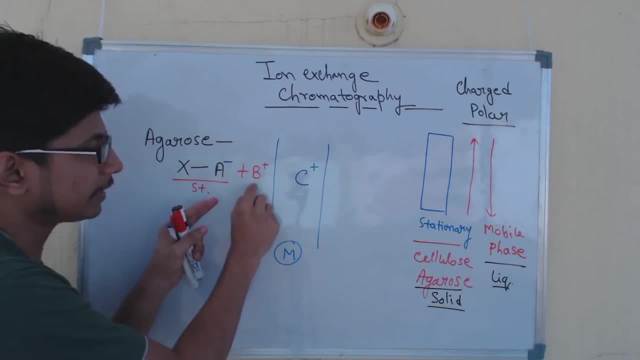 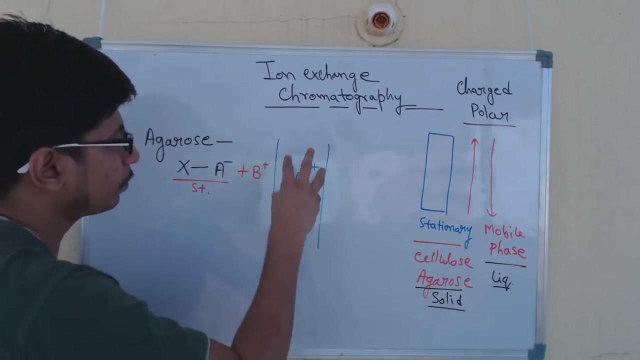 an ion- ok, and that ion is blocked by another ion of same type- ok, maybe it's a cation exchange, chromatography, what it means. this will exchange this cation for the other one. so let's assume here in this mixture we have both cations as well as anions. let's draw another anion. 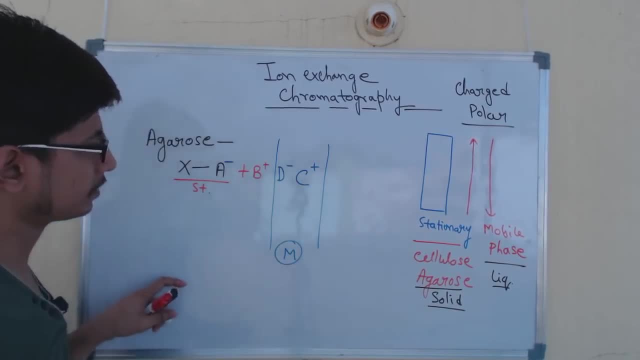 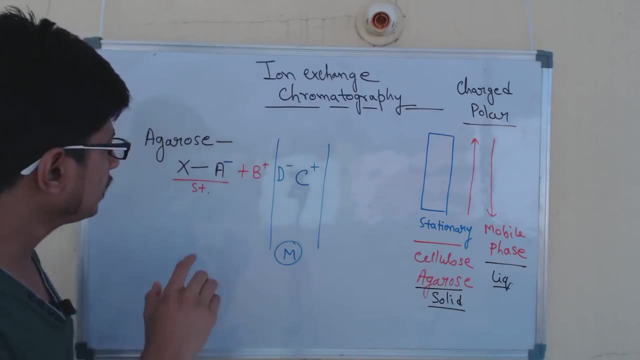 here. So we have a cation, we have an anion. this is the mixture. from this mixture we only want to separate cations, ok, and this is our stationary phase, where we have the agarose attached with the ion exchanging molecules, that negatively charged molecule which is fixed with this. 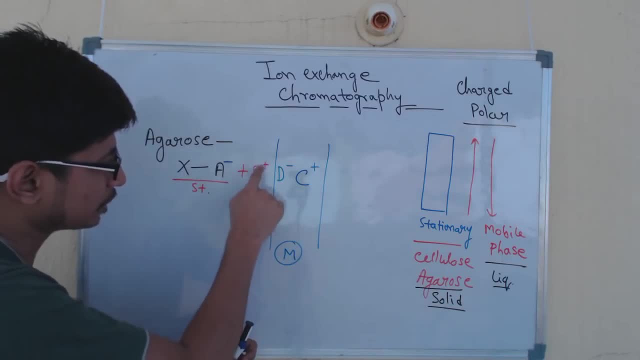 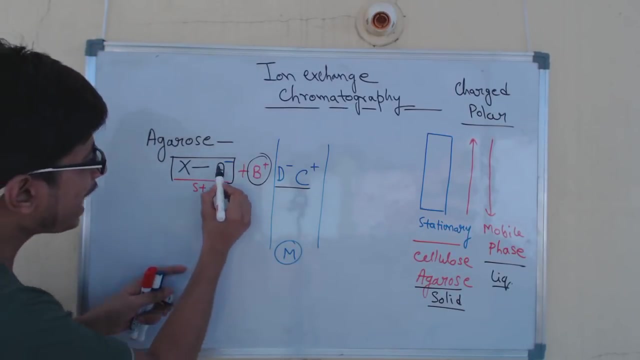 with this agarose as well, as we have a positively charged molecule which is masking the negatively charged molecule there. now the idea here is the exchange, How the exchange will work. remember, this part is completely fixed as stationary, so the exchange will occur between this and here right. so here how the exchange will happen. 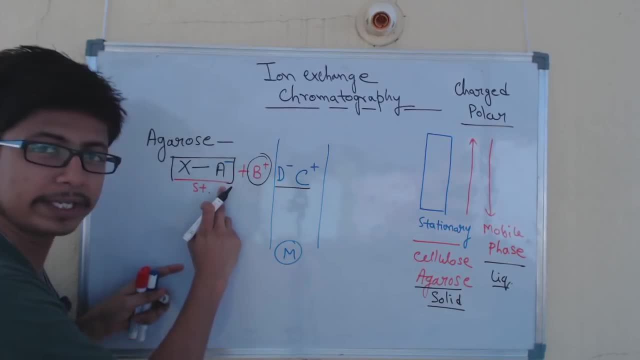 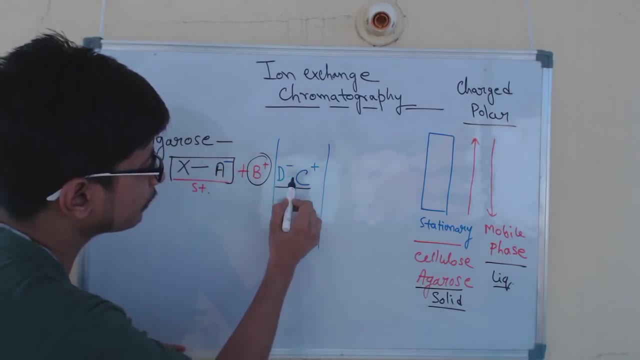 as this agarose is attached to a negatively charged molecule. negatively charged molecule will always try to interact with the positively charged ion. so among this mixture of negative and positive, This a will try to clear with C+ Instead Of D, Because D And A 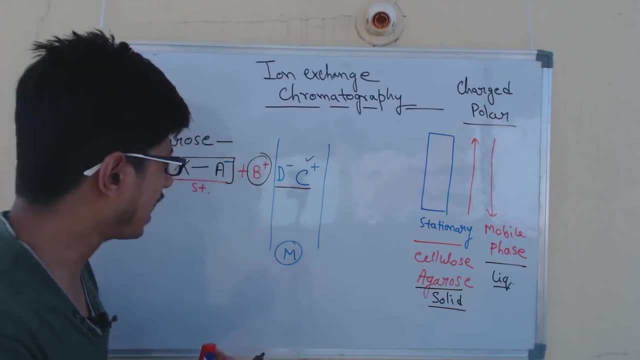 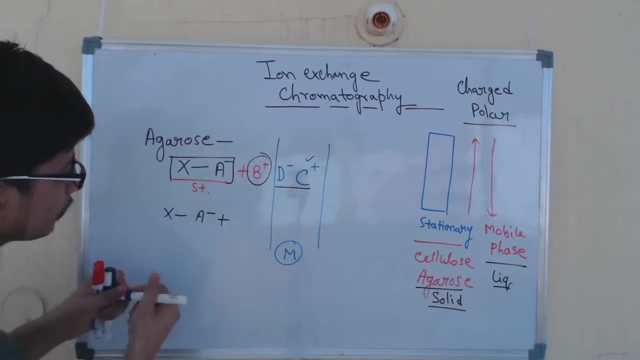 Is the same charge, They will repulse where C And A Opposite charge will attract. so after that what we can get is something like: this night will be attached with the C+. So now, in the stationary phase, we have C plus attached, while the B plus and D minus will. 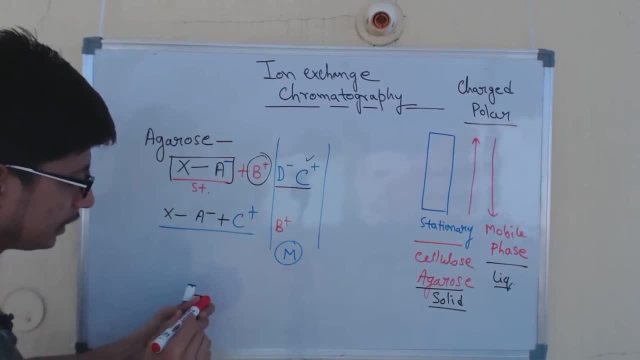 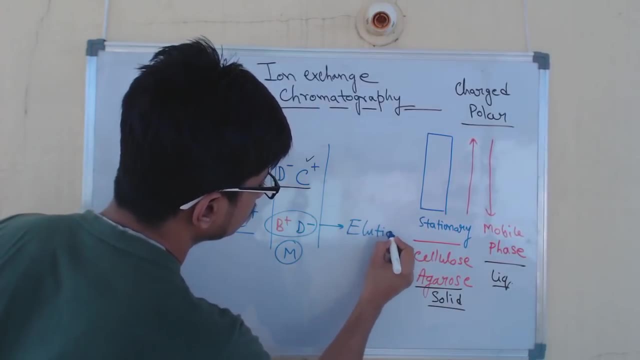 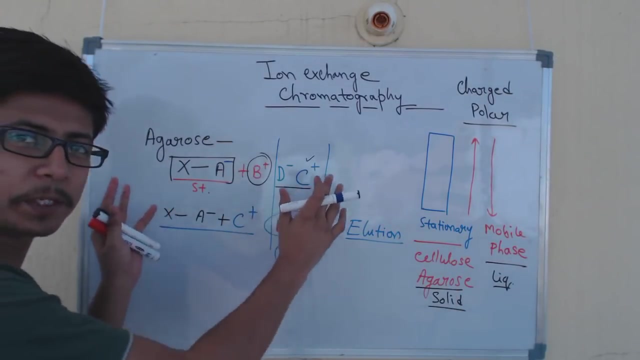 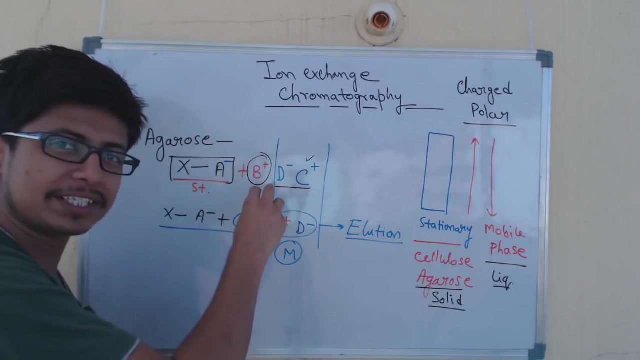 be now present In the mobile phase And this thing will be. This will be okay. so this is the idea, the big picture. this is how it works. ion exchange: that means there is I am present and there is one I'm attached and will exchange that. 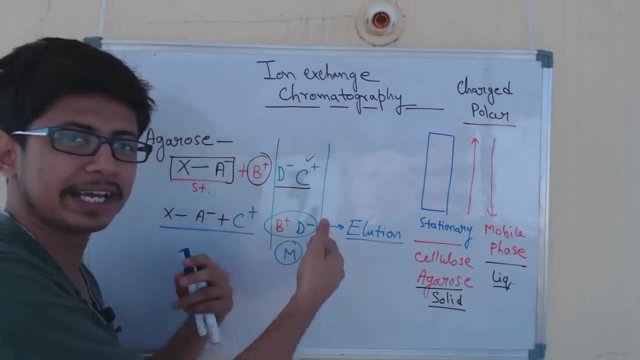 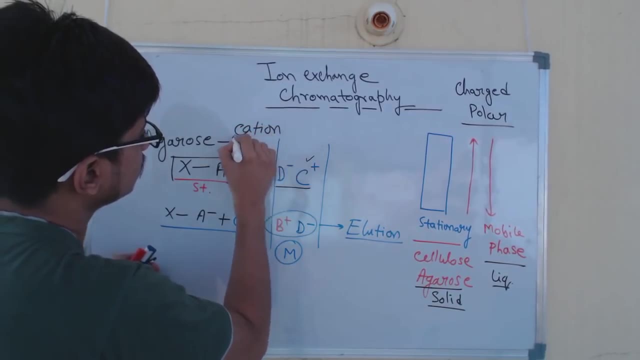 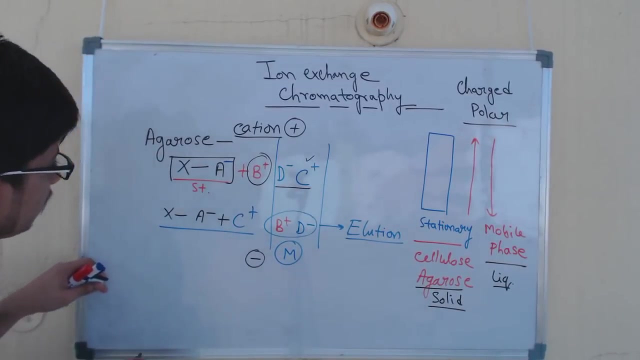 at a time for another ion that is in the mobile phase. that is the idea now. this is the cation exchange. Remember, it is a cation Exchange Which is positively charged- Look at for the anion exchange- or negatively charged, the case will be like this: 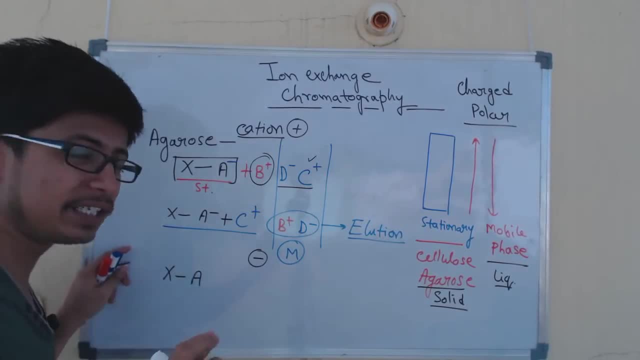 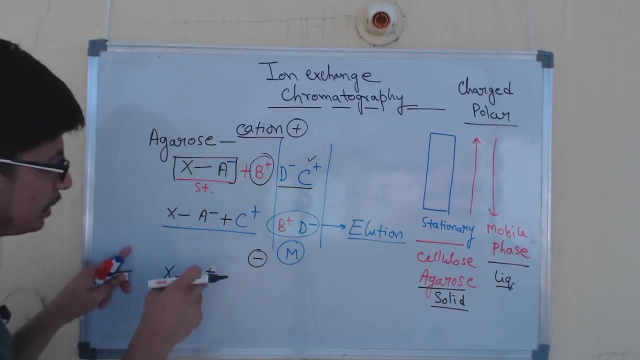 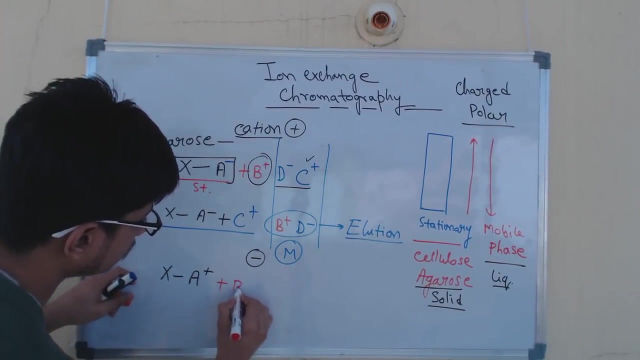 In the in the anion exchange chromatography, the raising. raising means the solid phase that is present in the column. that raising will contain positive charged molecules instead of negative, because yet they need to bind with anions, Okay, And then up At They also present a negatively charged attached to it. and then in the mobile phase, 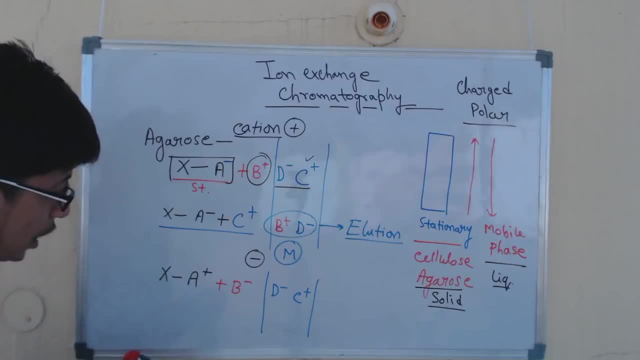 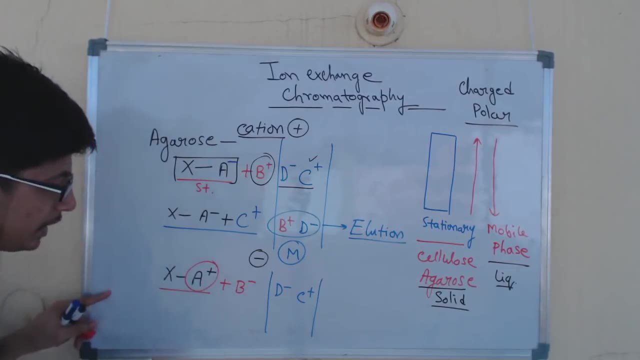 Let's say same things are present in the mobile is D minus and C plus. So now, what we know as this is the stationary phase, the fixed phase, and it contains a positive charged ion. it will interact with this negatively charged ion in the mobile phase. 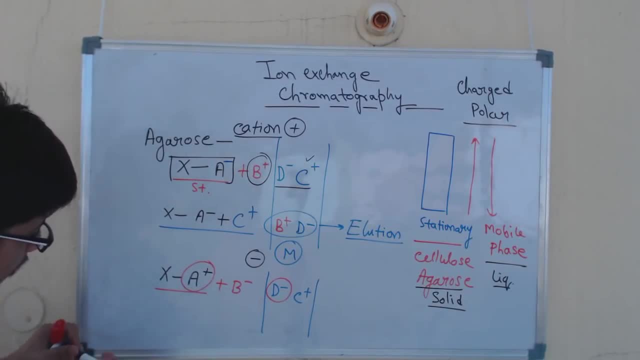 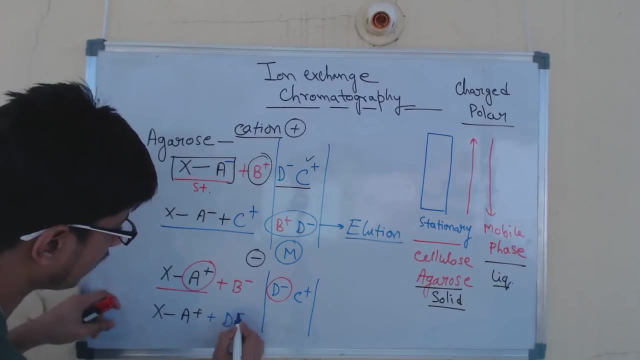 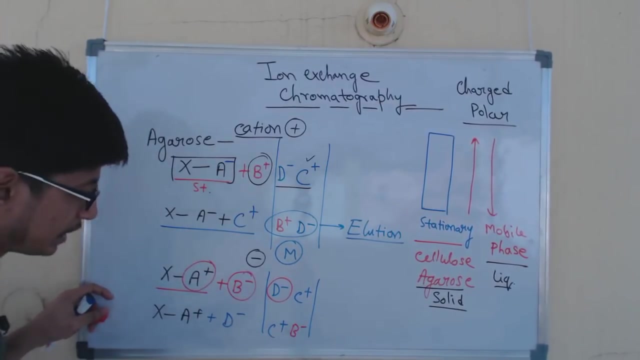 So now the pairing will look something like this: A plus. along with that, We will have this D minus, while the C plus and is B minus. this is the and it will come to the mobile phase. So remember this D minus will attach to the a similarly here, as is negative C plus attached. 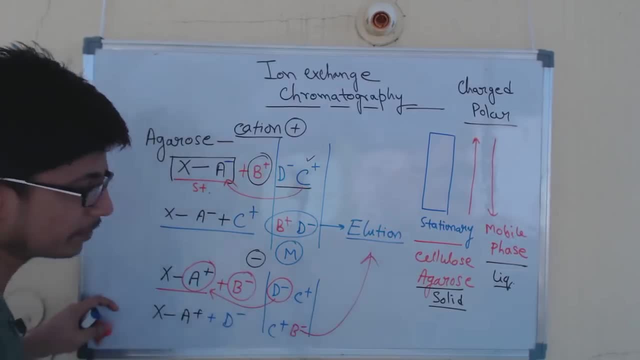 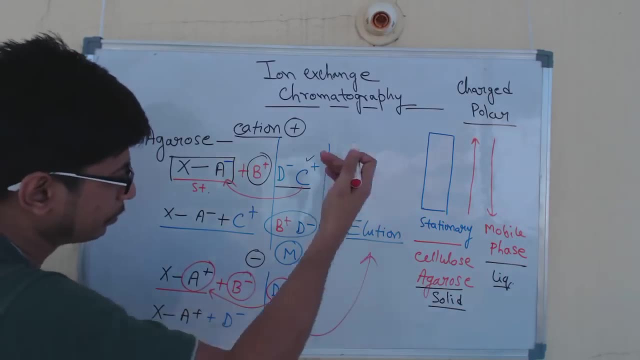 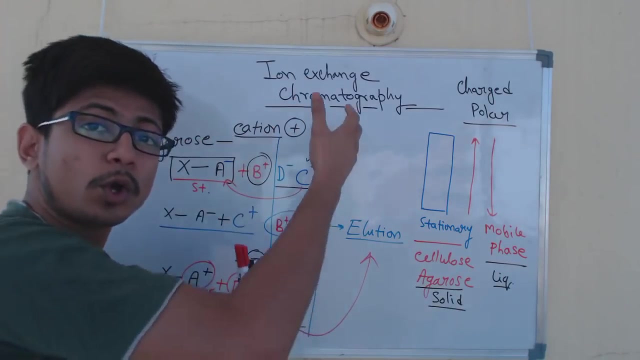 to the, so, ultimately, at after that, it will be eluted. So this is the idea. Okay, It will be removed. not actually illusion, It's not an illusion or removal. After this removal is done- Remember, after running this whole system, after running this whole process, whole column. 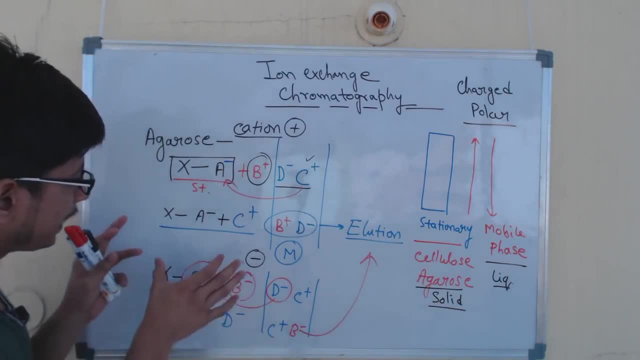 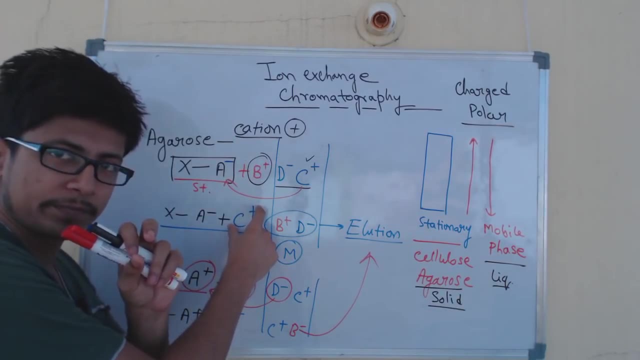 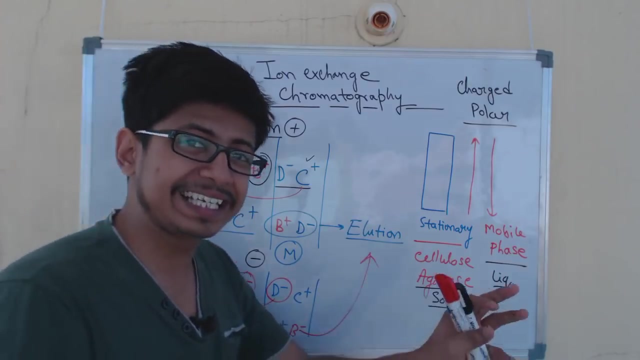 with all the solutions and molecules, what we will get. we will get some things like this, where we have the agarose bind with our molecule of interest. okay, now all the unbound molecules are washed away with buffer solution. once that thing is done, then the idea is to separate. 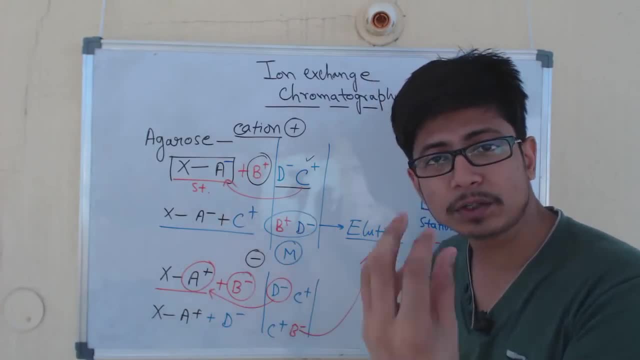 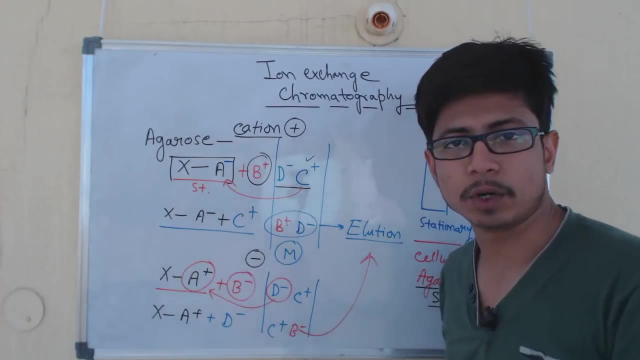 these molecules independently, Because we want them. We want to fish them out from the mixture of other ion molecules. So then, after that, what will we do? we exclude these molecules. that process is also known as illusion. okay, and how we do that? we simply increase the concentration of same type of. 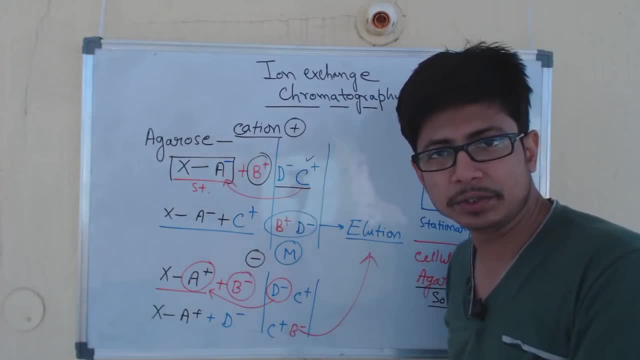 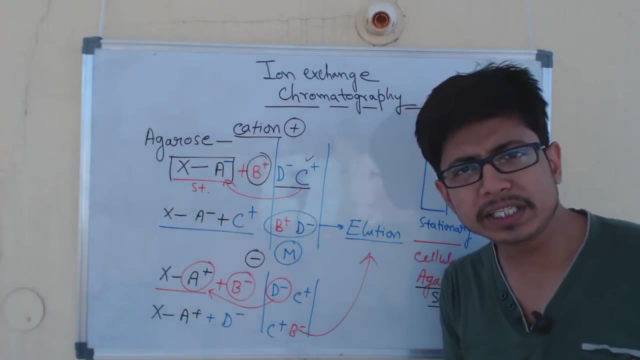 or same charge ions in the buffer. in the solution We increase the same charged ions. okay, for example, here we need the positive charge ion to elute this one- So It is a particular positive ion concentration- hugely so that those ions start to bind with. 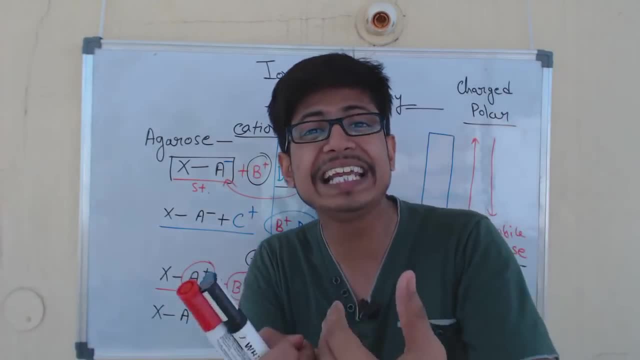 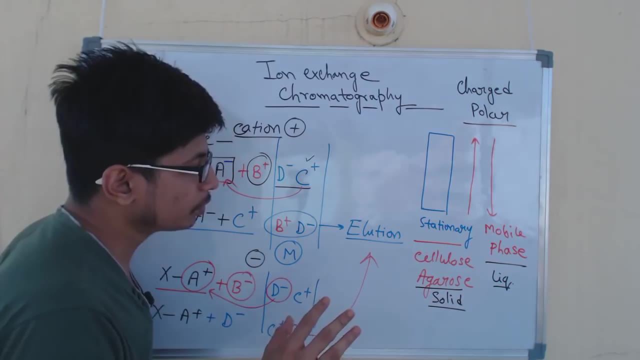 this and see start to come out. This is the way we elute things. so for any chromatographic reaction that you want to see in future, keep three things in your mind. first thing, you need to know about its stationary phase. then you need to know about its mobile phase and how they interact. second thing is: 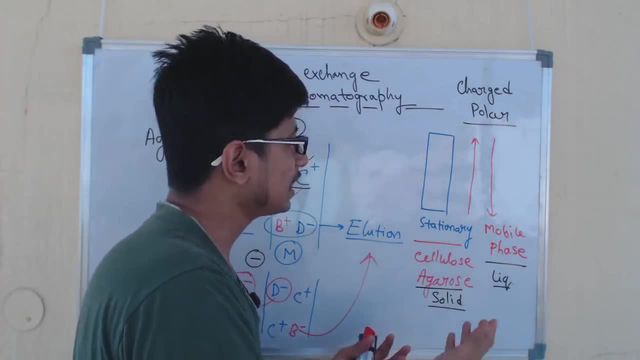 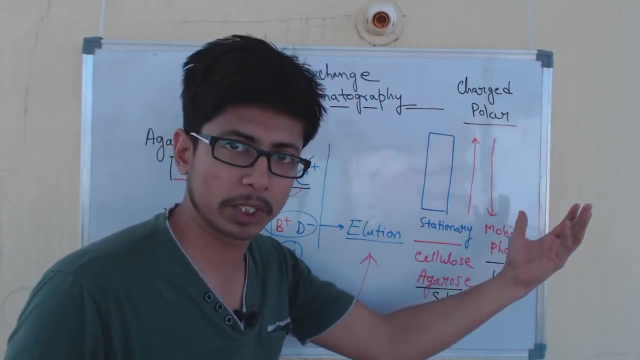 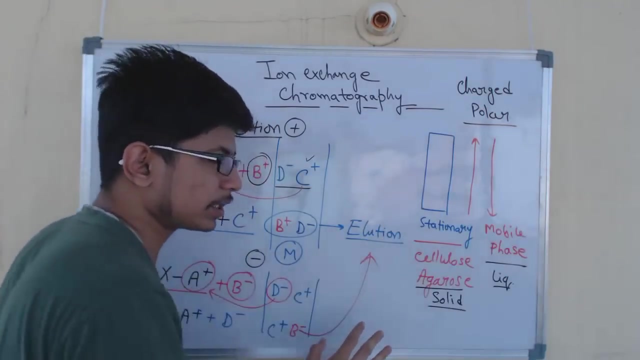 that what kind of solvent they are using for this process. like in this case, we use aqueous molecules. In this case, organic solvents are generally not being used, though we can use this process for many different varieties that I'm going to talk to you later, but this is the idea. 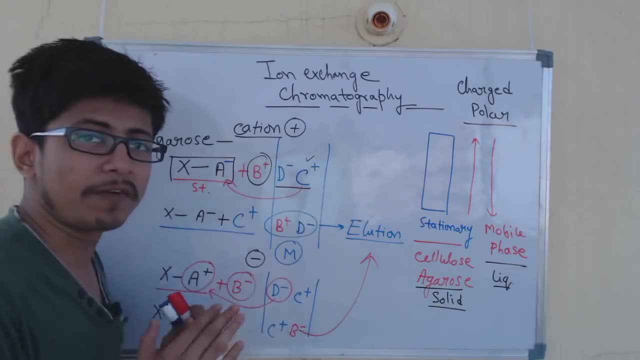 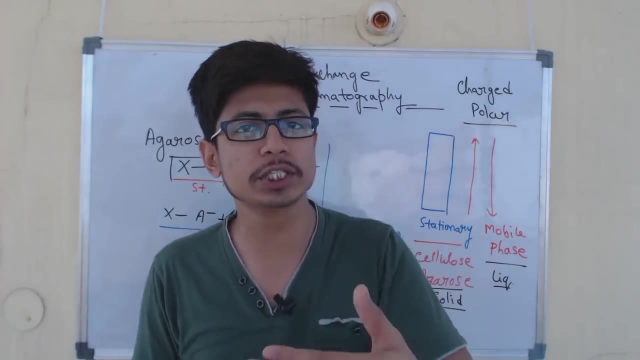 this is the first thing you need to know. the second thing you need to know is the principle of how it's working, how the separation working in big scale, and the third thing you need to know is how the illusion take place. that is, how you separate your target molecules. 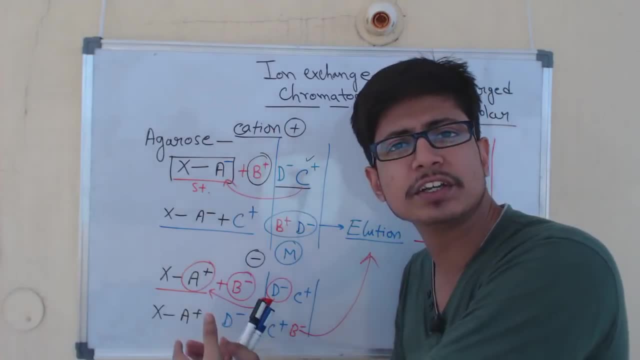 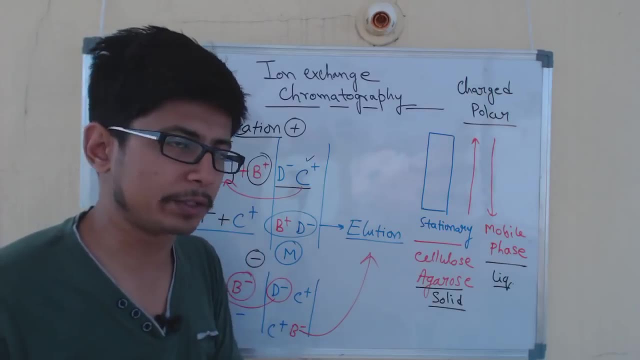 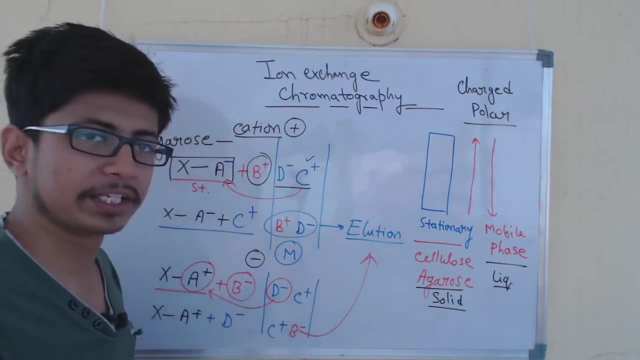 From Binding or from from the stationary phase after the chromatography is complete. so once you know three things, you know the complete overview of that chromatography. as I told you all these three things, now it's time to talk about the advantages and disadvantages of ion exchange chromatography. that one is that an exchange chromatography works for. 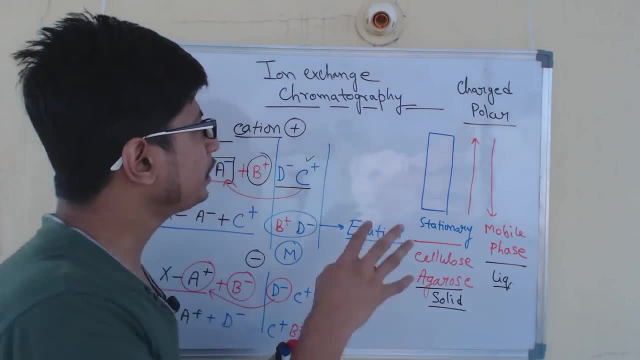 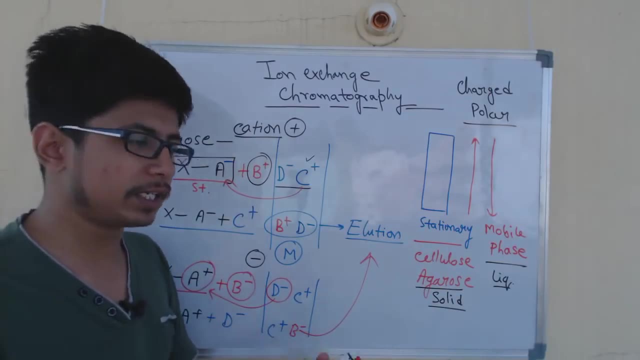 polar molecules and charged molecules very well, and we use an exchange chromatography in the field of water testing plants. Well, You need to check for certain water or waters, dissolved molecules and separate them from each other. so it's used in water testing labs in, you know, in different wastewater treatment. 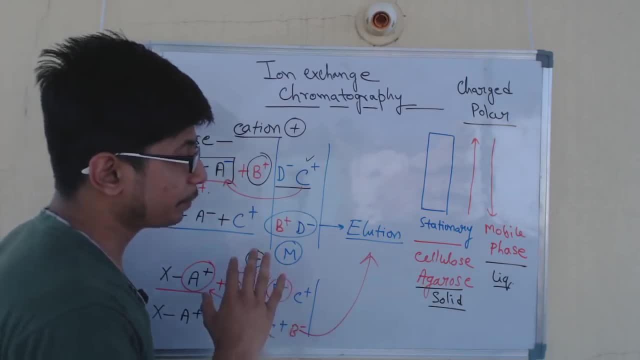 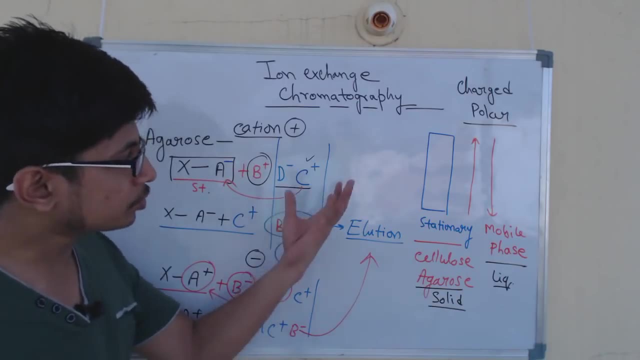 plants and stuff. second thing: we can use an exchange chromatography for separation of proteins, for example. we can use it for the separation of hemoglobin as well as different for fighting. we can also use it for the other, for fighting ring containing molecules, for example, like chlorophyll also. 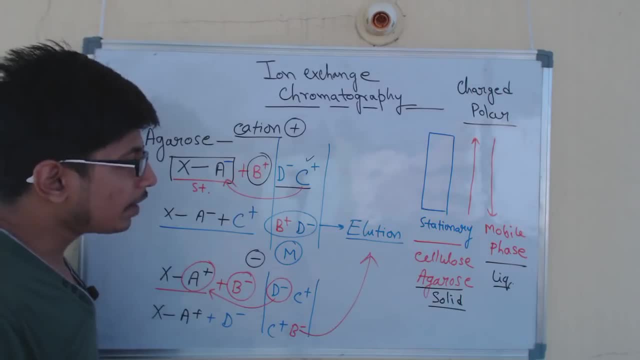 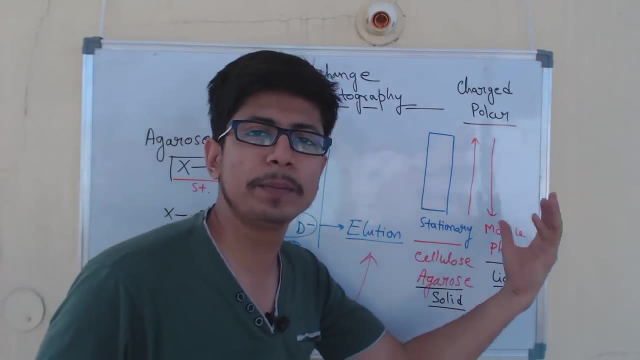 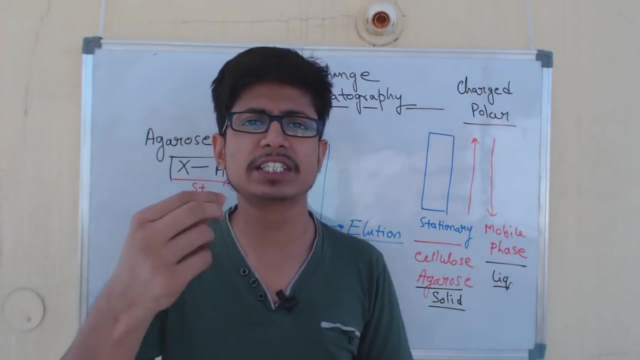 So these are the advantages of an exchange chromatography. however, the disadvantage is that in this type of technique we cannot use a though those hydrophobic molecules for the separation. it only relies on the charge. and as it is relying on the charge, a single charge change can cause this whole process to change and alter. you know an amino acid in a protein. 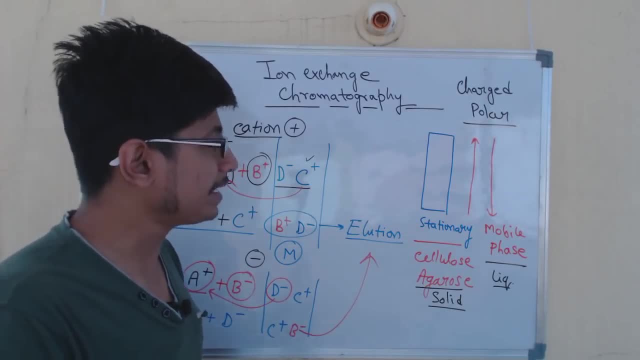 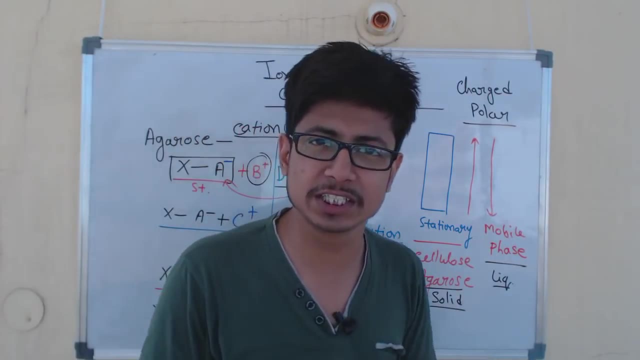 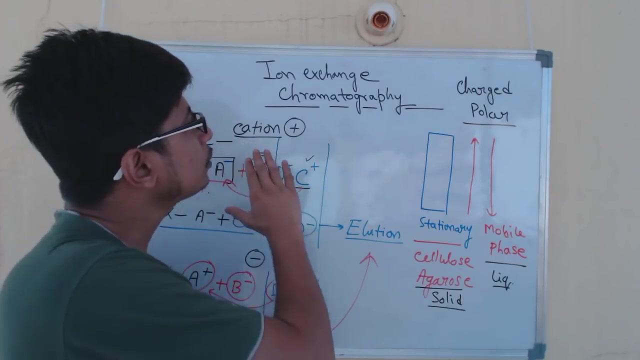 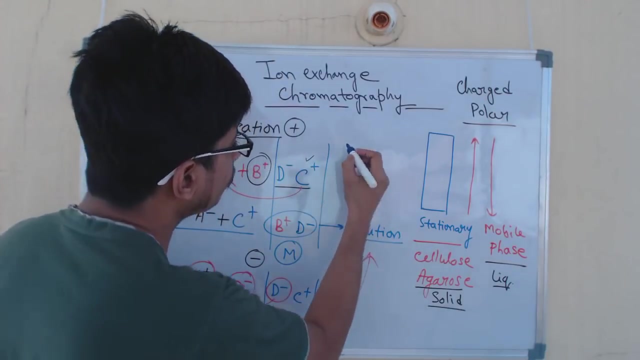 is consisting of many different types of amino acids, right, so all these amino acids have a different charges. right now, if one of the amino acid charge changes, that will ultimately change the overall charge of the protein and that will affect in the separation of that protein using an exchange chromatography, and this is also known as electrophobic, a chemo. 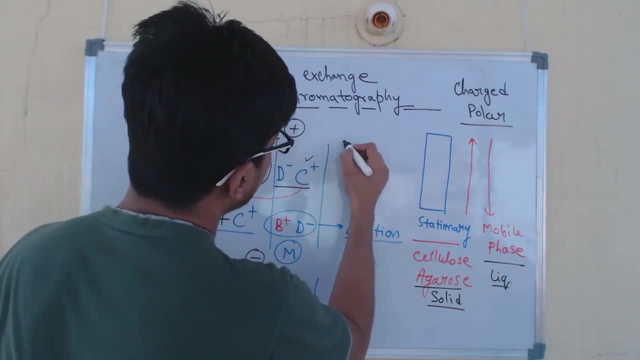 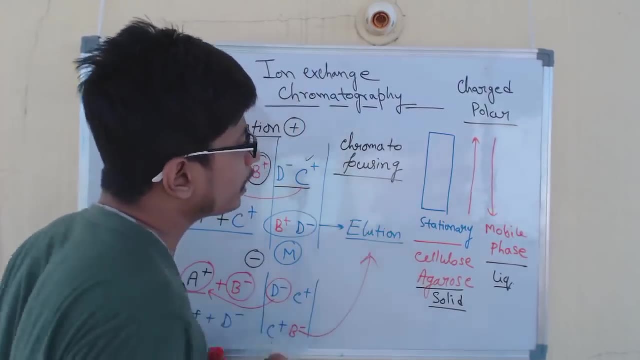 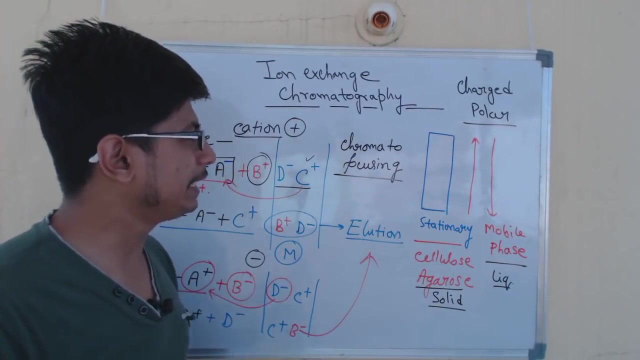 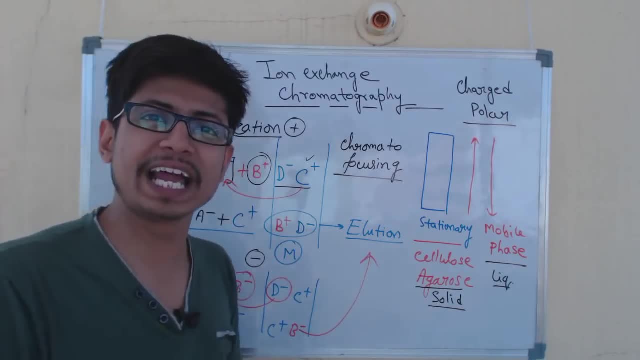 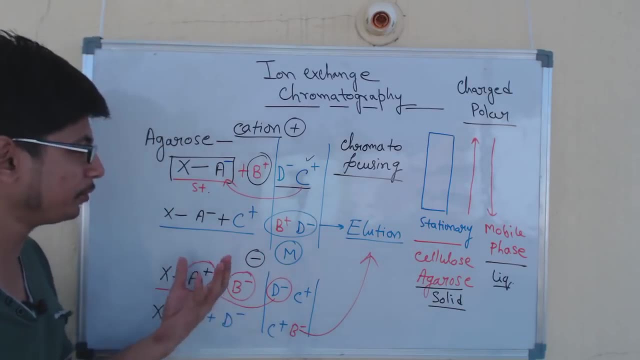 charge. we can modulate the illusion of that molecule using an exchange chromatography- see the, because you know this illusion is very, very important- how you ultimately get the new tent and the molecules at the end, because you need to have all these molecules at your hand. 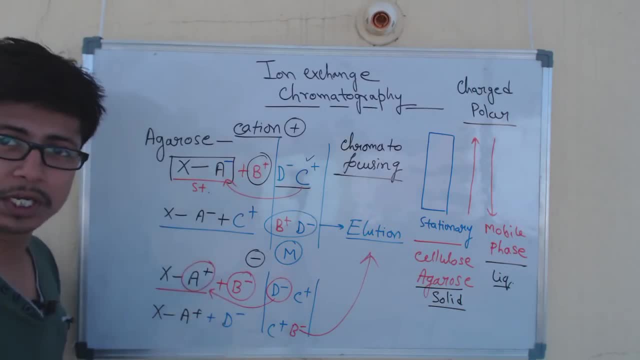 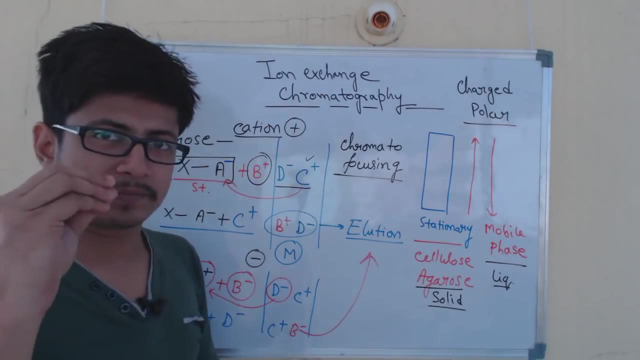 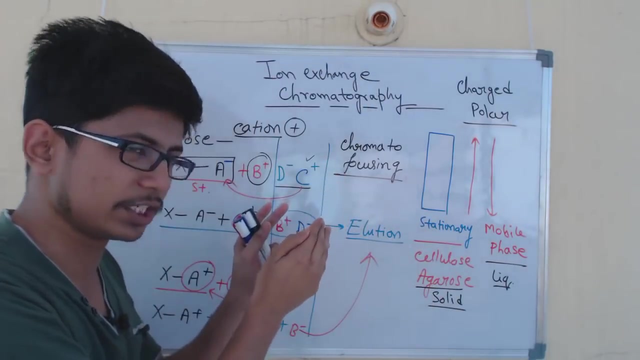 That's your idea. You need to purify it and then you need to use it for your purpose. so here that is called as a chromato focusing steep. okay for focusing a specific charge, or focus on a process where we get a specific charge molecules there and by changing the charge you can get the details. 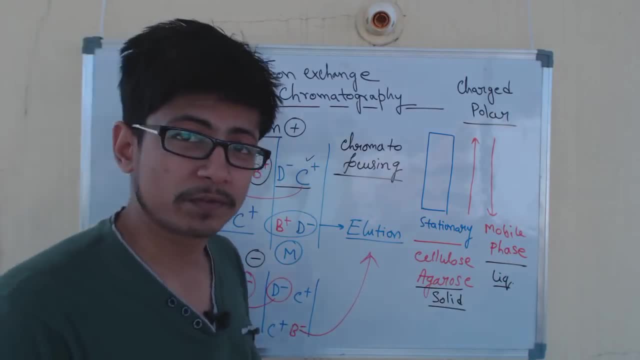 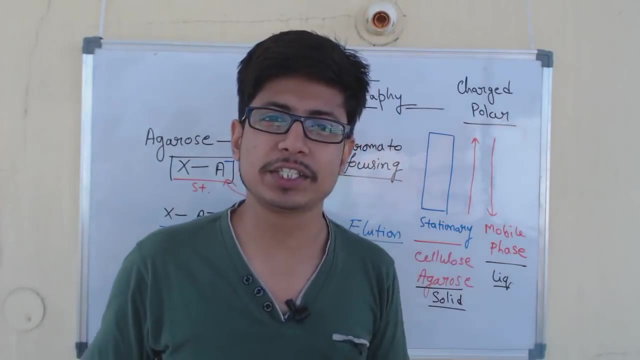 by changing the charge you can get that molecule out from the column pretty easily. that is the idea about the An exchange chromatography. I hope you understand an exchange chromatography. if you like the video, please hit the like button. share this video with your friends and definitely subscribe. to my channel to get more videos like that. thank you.